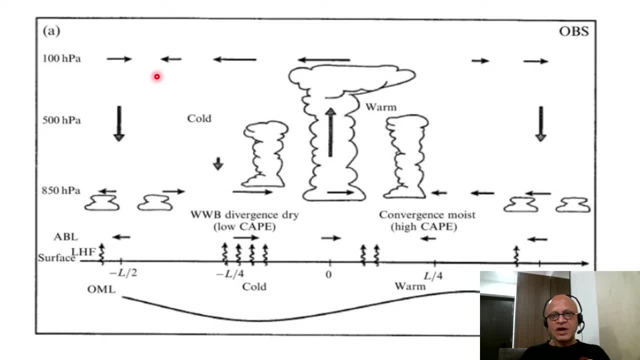 but you diagnose the full coupling that's there to see at intra-seasonal timescales. what are the cloud SST feedbacks in those models and cloud wind feedbacks. And then there is a lot of work recently showing that specific improvements in convection representations like dilute plume approximation- 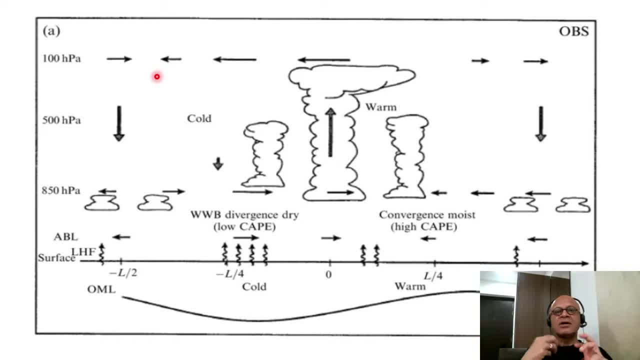 if you don't know what that means, don't worry about it. Convective momentum transport, again: if you don't know what that means, don't worry about it. So those kinds of things are shown to improve the coupling nature of the MJO's ocean-atmosphere interactions. 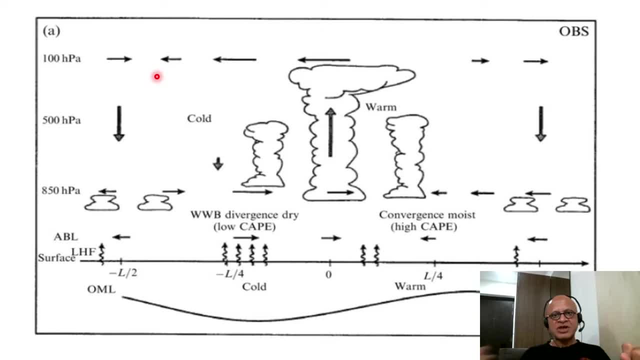 and improve certain aspects of the MJO's, like propagation speeds and structures and so on. But in this context here we start with looking at the vertical structure of the MJO. so you have the deep convection here with the shallow congestus on either side. 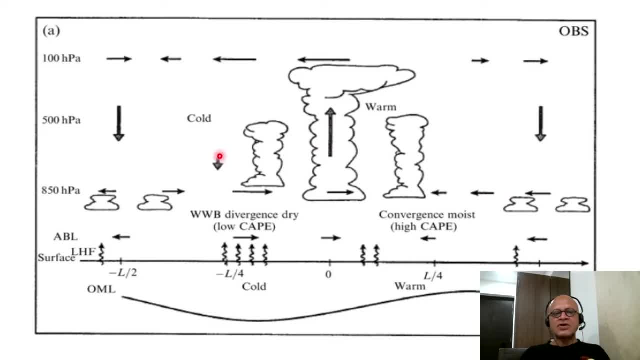 and so you have strong vertical motion here and weaker downward subsidence here and stronger subsidence away from it. so you have the convective complex, as we have called it, and there are the shallow cumulus, and all the processes we are looking for exist here. 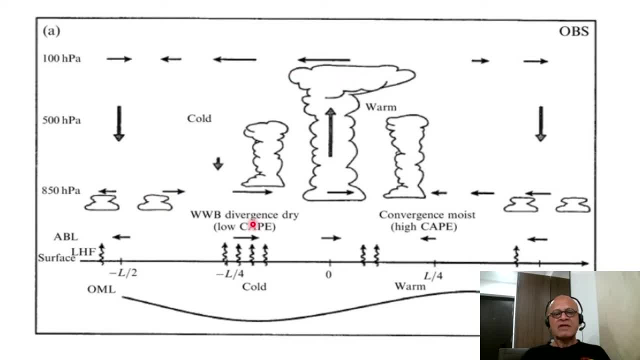 so you have strong easterlies in the upper level and westerlies at the lower level, and in the 850 hectopascal, which you can think of as the top of the planetary boundary layer, there is the westerlies on the western surface. 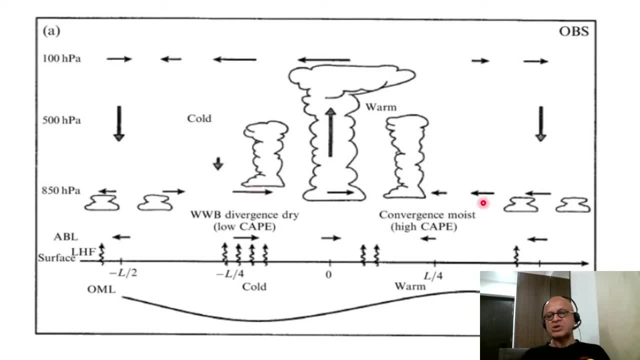 on the western side of the MJO convection and easterlies on the eastern side and similarly at the lower level, and this is the atmospheric boundary layer. So you have warm and cold temperatures in the atmosphere, you have latent heat flux. 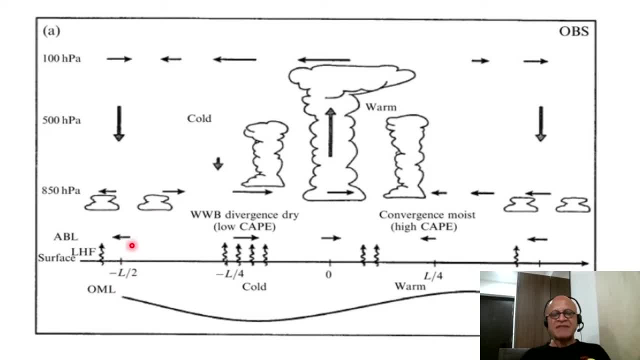 where we have to consider the impact of the MJO-driven winds on the background winds to see where latent heat flux is. latent heat flux is enhanced to cool the SSDs and create ocean mix layer response, so you have a deepening of the ocean mix layer here. 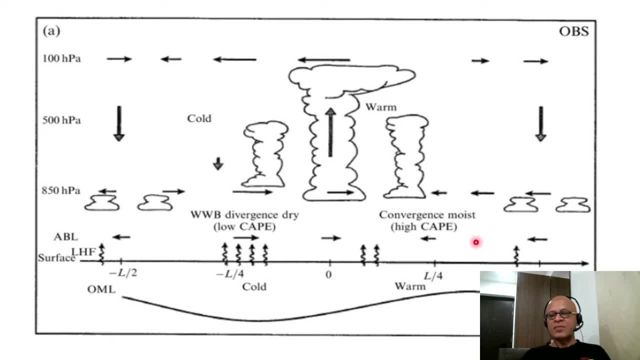 ahead of it, you have a weakening of the background winds, assuming they are easterly- which we already said are not easterlies- in the Indian Ocean and in the Western Pacific. nonetheless, this is the kind of model we always use for vision. 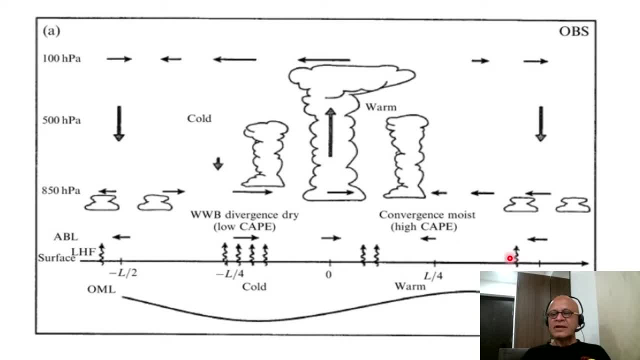 so you have reduced latent heat flux and warmer SSDs and shallower mix layer here. so now you have feedback from the ocean to the extent that the stronger winds behind not only increase latent heat loss, which you had invoked before, but also you have ocean mix layer processes. 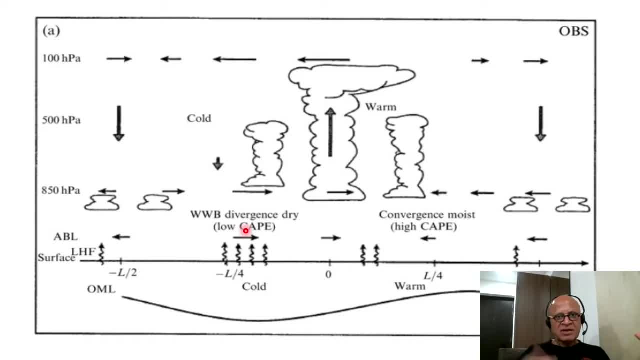 where you have entrainment and cooling and deepening. so to deepen the mix layer you need turbulent kinetic energy, which is cube of the wind speed, and cooling, so you have entrainment of colder water, and deepening, so deepening means you are chewing into the colder water below, and so on. 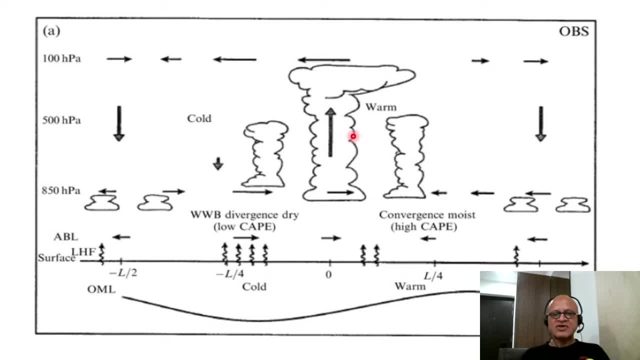 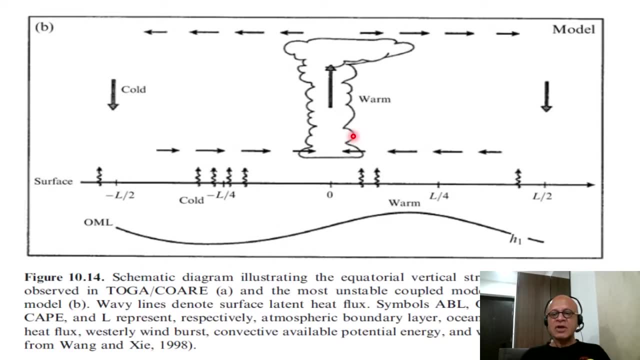 so this is the general ocean atmosphere interaction within which the instability, the growth growing mode and the most unstable coupled mode are looked at in this model, which I am not listing the equations of the model and so on. it's not perfect. 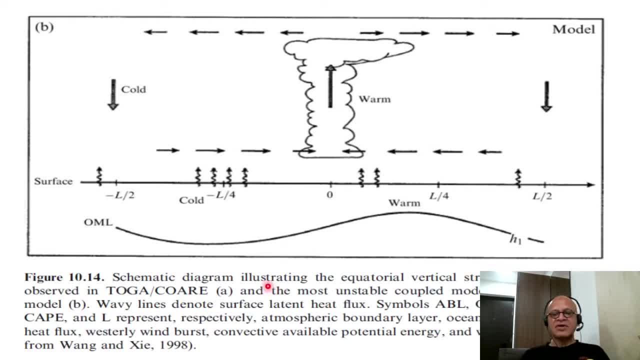 it has issues. but here is a schematic diagram that we looked at for the MJO structure, and in B we are looking at the most unstable coupled mode in the theoretical model. wavy lines denote the surface latent heat flux, which is what we already looked at. 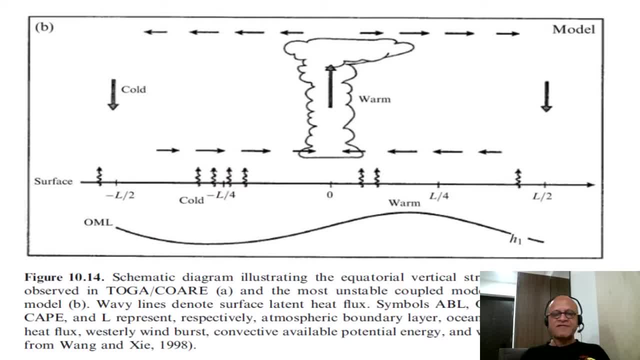 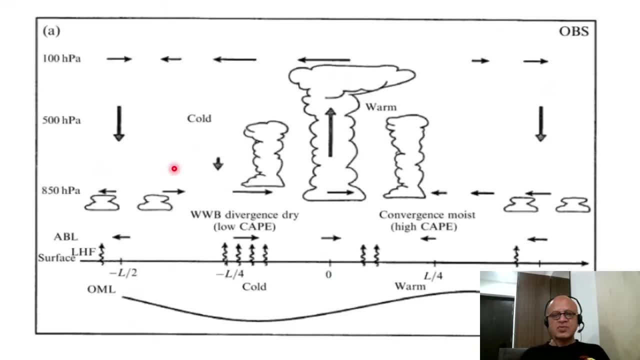 and ABL, OML, LHF, WWB, KPI and L represent respectively atmospheric boundary layer, which you already know here. CAPE is the convective available potential energy. WWB are westerly wind bursts, so those are at a certain synoptic scale. 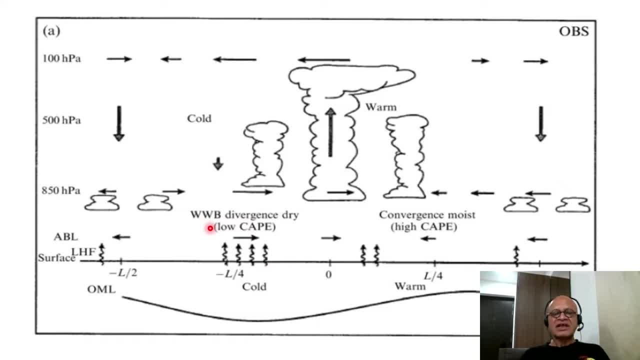 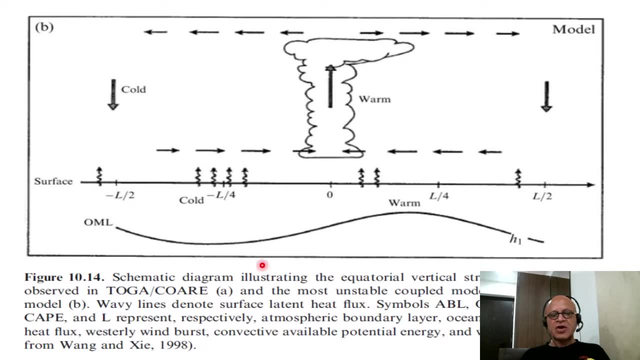 with a certain wind speed of 7.5 mps and they last for about a week and they send off Kelvin waves in the ocean, can cause remote responses in the ocean ahead of the MJO, and so here any additional thing we have to look at. 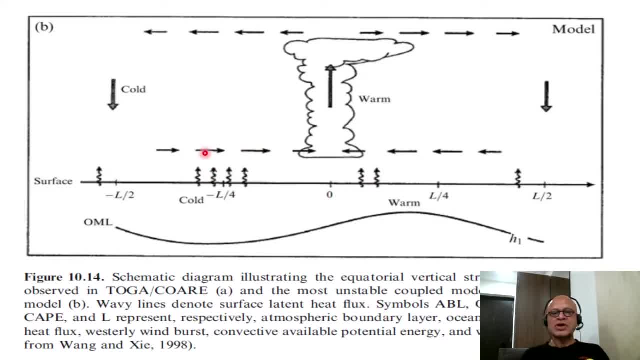 so the most unstable mode here is showing again the strong convergence in the free into the deep convection and you have the strong divergence at the upper level, strong vertical motion and the subsidence ahead and behind with the increased latent heat flux. 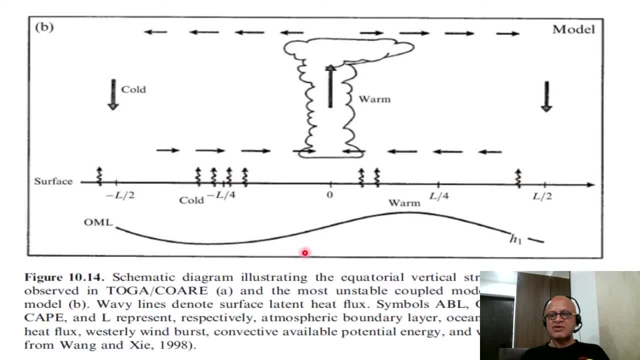 and decreased latent heat flux, here with the mixed layer response, and the model has a equation for computing H1, the mixed layer depth in terms of the winds, entrainment, mixing, parameterization and so on and so forth. 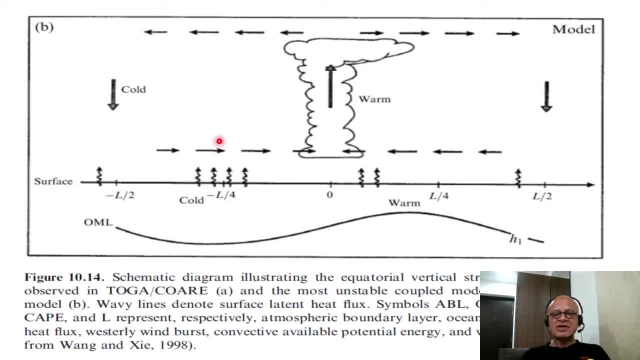 and this is typically what is done, but in the real full GCMs, whether it's a forced ocean GCM or a coupled GCM- what is not clear is what we talked about before in terms of low frequency rectifications. 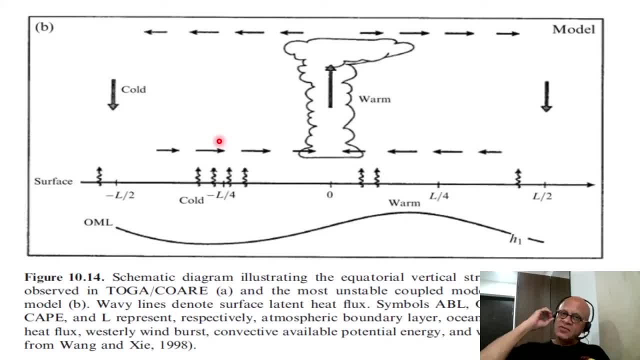 for example, as I said, the westerly windbursts associated with the MJOs send off Kelvin waves and typically westerly- I mean westerly- windbursts always produce a downwelling Kelvin wave. 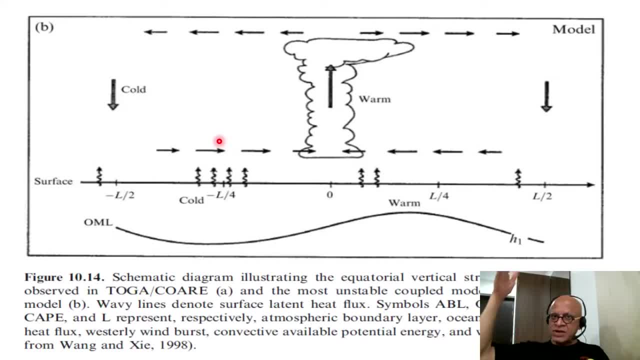 which would push the thermocline down, weaken the stratification and with the same TKE. in that case you can deepen the mixed layer and increase the heat content ahead of convection and if you have multiple MJOs. 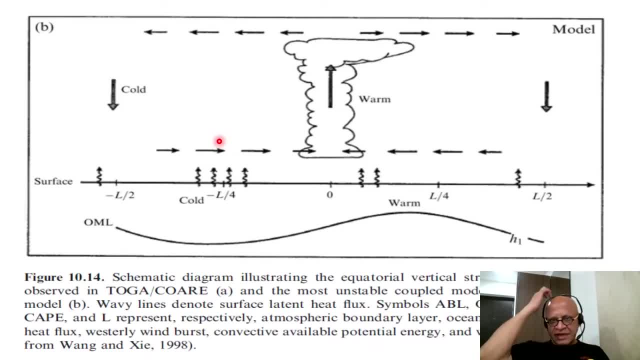 it's been shown with models that the mean state of the ocean changes, so multiple westerly windbursts would leave you with, let's say, a deeper mean mixed layer at lower frequencies, even at a seasonal time scale. 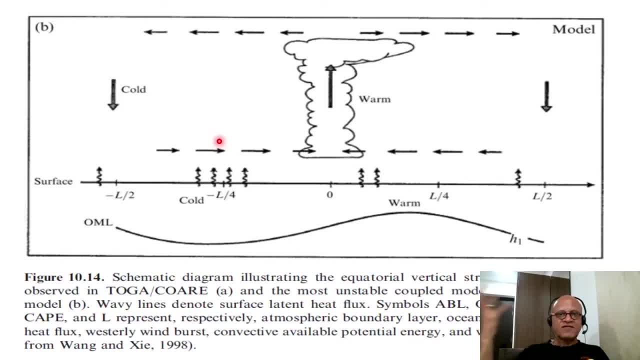 okay, and that would also show up in terms of chlorophyll response in the ocean, because every time you have entrainment and mixed layer changes, you're entraining nutrients into the euphoric zone where there is chlorophyll blooms. 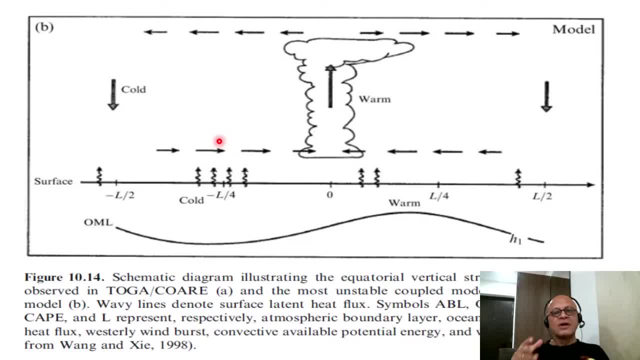 and there is a chapter in the book at the end talking about biological responses which I'm not going to go into in this series. but that also shows that there are low frequency rectifications associated with these MJO related winds. 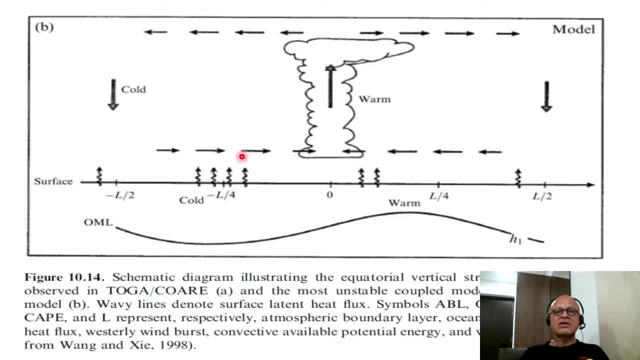 what do they do in terms of the seasonal variability of the MJOs, or does the MJO that get organized after the first MJO somehow benefit from the signature in the ocean heat content created by the first MJO? 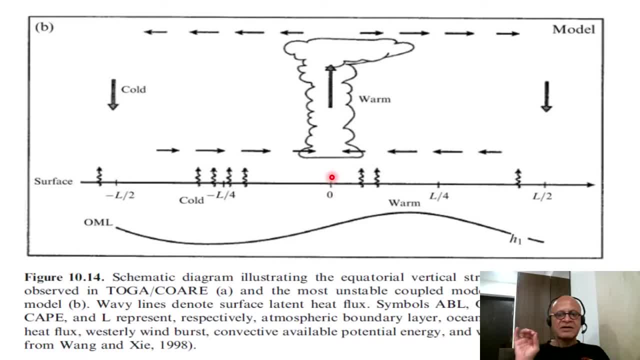 or is that a negative feedback? and all those sorts of questions have remained which we are not getting into here. but there are papers which show that the equatorial Kelvin waves generated in the Indian Ocean hit the coast of Indonesia. 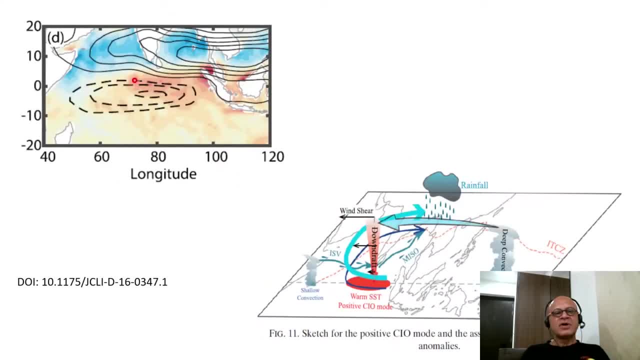 I don't know if I have a map. yeah, so let's say Kelvin waves are generated as the MJO is traveling, propagating eastward and it's generating waves along the way. those Kelvin waves go off into the Bay of Bengal. 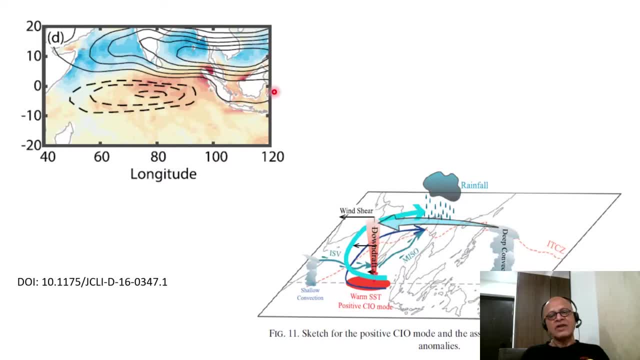 and down Sumatra into Java and so on, and there is the Indonesian through flow coming here together that generates some interactions here and baroclinic and barotropic instabilities, depending on the season. 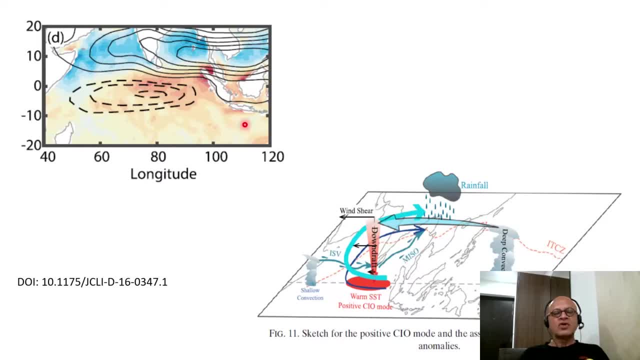 boreal summer, boreal fall and so on. those instabilities then generate waves which can go back and affect the MJO genesis region and also send off Ross B waves that affect generally the. 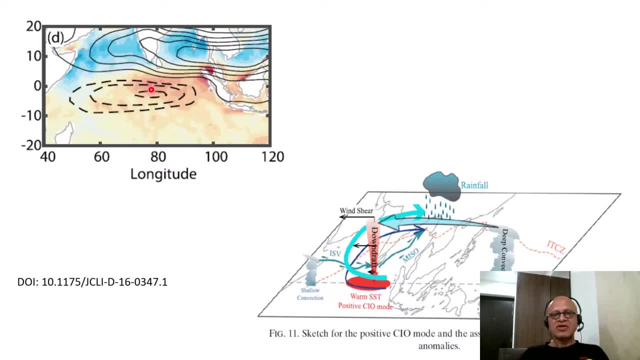 AC interactions, vertical structure and so on here, depending on the season. so when we talk about ocean atmosphere interactions, those kind of things are also important. but in this case of ISO theories obviously we are only looking at. 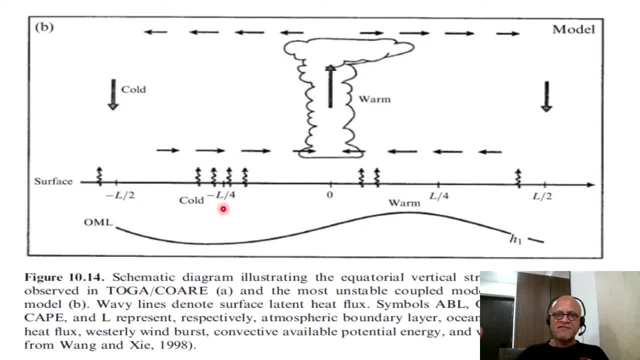 MJO- one MJO and not the lower rectification, low frequency rectification and impacts on other MJOs. so to the extent that we are looking at just one MJO, it is clear. 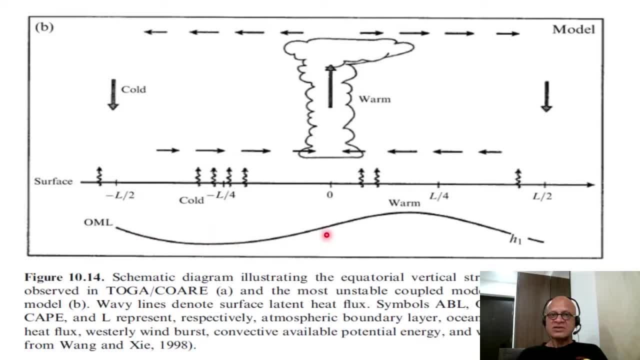 that the ocean mix layer processes. so ocean dynamics are involved in the MJO, as well as the ocean atmosphere interactions which we talked about before in terms of just enthalpy exchanges or heat flux.